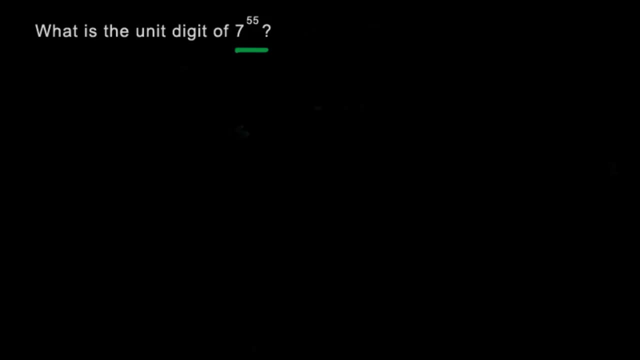 problem, This problem, what makes it approachable, is that we're only looking for the units digit right here. So let's make a, let's consider a table, Let's think of a table where you have a number 7 to the power of n. This column is going to be n and this is going to be the unit digit. 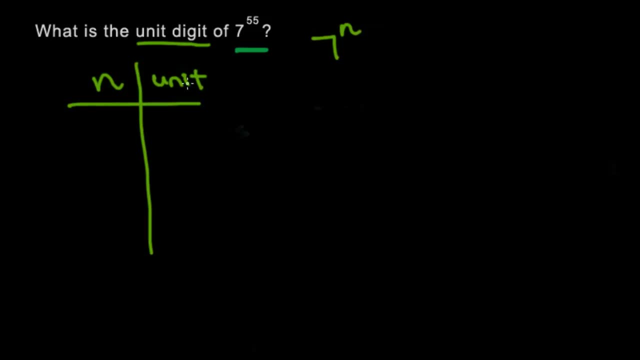 of 7 to the power of n. So when n is 1, it's just 7 to the power of 1,, which is unit digit is 7.. And if n equals 2, it's 7 times 7,, which is 49. The unit digit is going to be 9.. 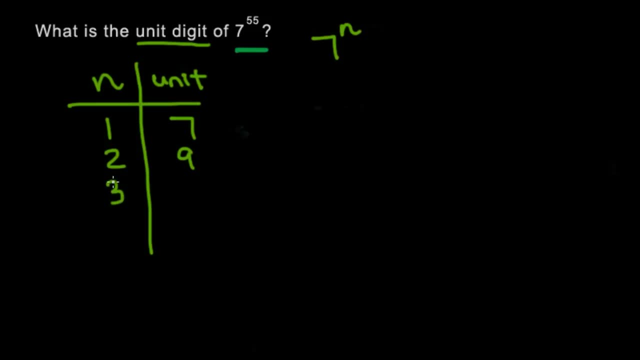 And let's keep going. 7 to the power of 1.. 7 to the power of 3 is 243.. So you need to just going to be 3.. And 4, it's simply just going to be 3 times 7, which ends in 1.. And let's just do a couple more values. 5 is going to be 7 to the. 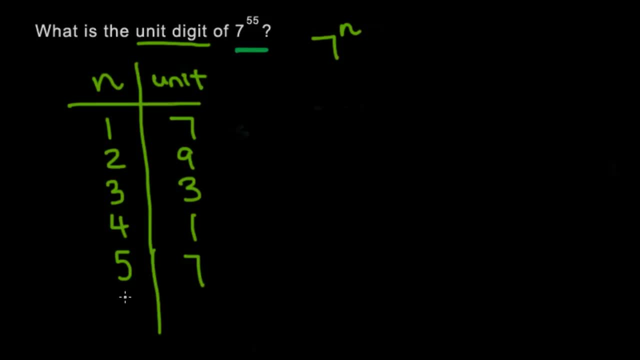 power of 5.. It's just 1 times 7,, which is 7.. And just one more: It's going to be 7 times 7,, which ends in 9.. So you probably noticed while I was writing this table. 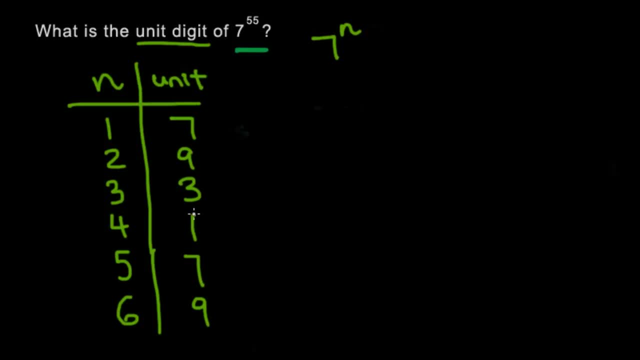 that the values repeat. So 7, 9,, 3, 1.. 7, 9 is going to be 3, 1.. 7, 9,, 3, 1,, just like that. So the value, the unit digit of this number, 7 to the power of n, repeats every four numbers. 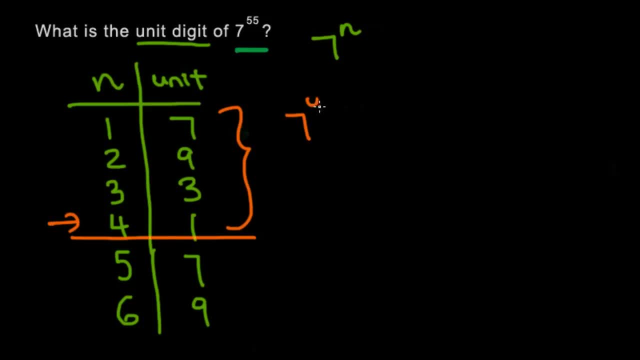 So what this means is that 7 to the power of 4 is going to end in 1.. 7 to the power of 8 is going to end in 1.. The same with 7 to the power of 12,. 7 to the power of 16,. 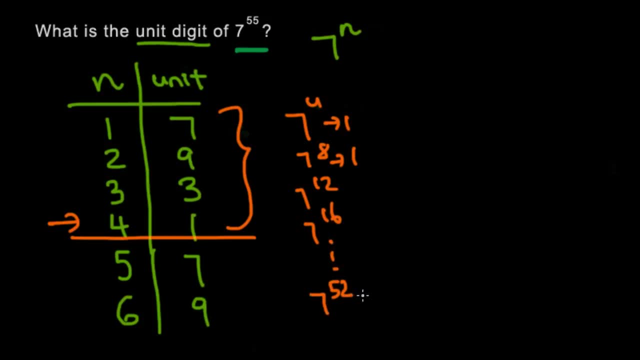 all the way up to 7 to the power of 52. It's all going to end in 1.. And that's because all these numbers, they're multiples of 4.. So we know that 7 to the power of 52 is going to end in 1, which means that 7 to the power of 53. 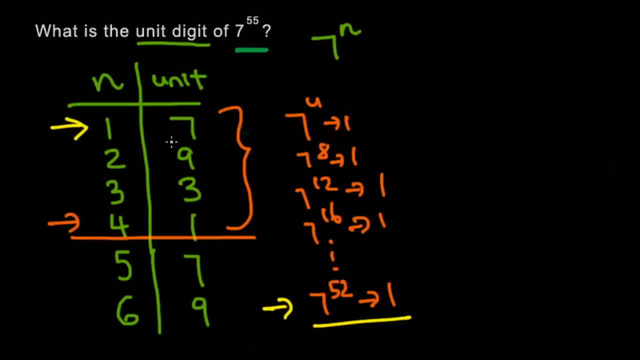 will end in 7, because you're multiplying one more 7.. And then 7 to the power of 54 will end in 9.. And then, finally, what we want, 7 to the power of 55 will end in 3.. So we know that the answer.